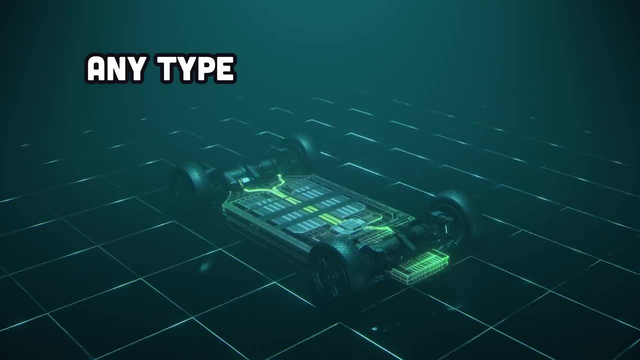 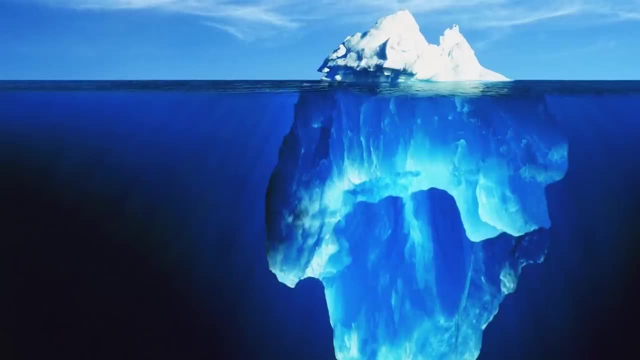 Nuxt, a batteries included framework for building any type of web application you can imagine with Vuejs. The purpose of Vuejs is to build front-end user interfaces with JavaScript, but a true full-stack web application also needs to deal with routing data fetching. 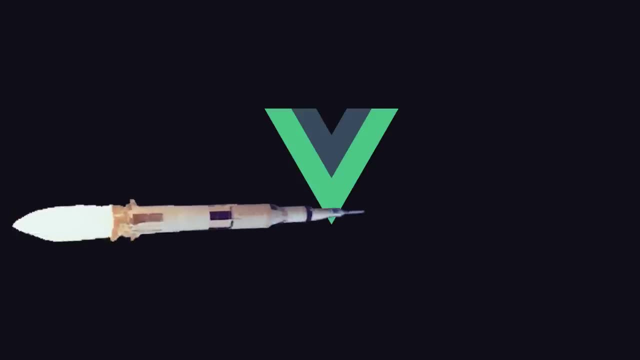 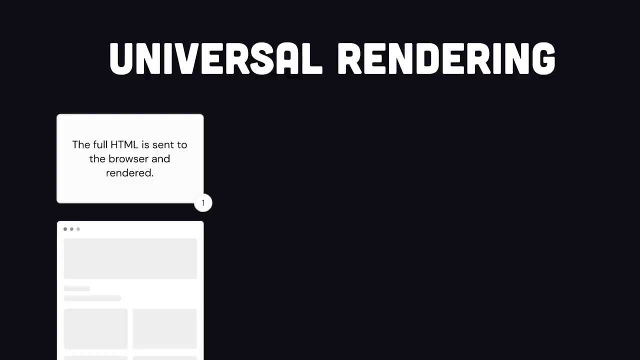 caching, deployment and more. That's where Nuxt comes in. It works by strapping its Nitro Server Engine 2 view, enabling multiple rendering modes from a single application. By default, it does universal rendering, where the initial page view is rendered on the server. 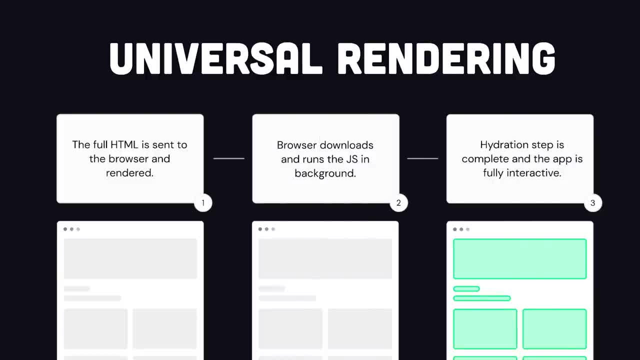 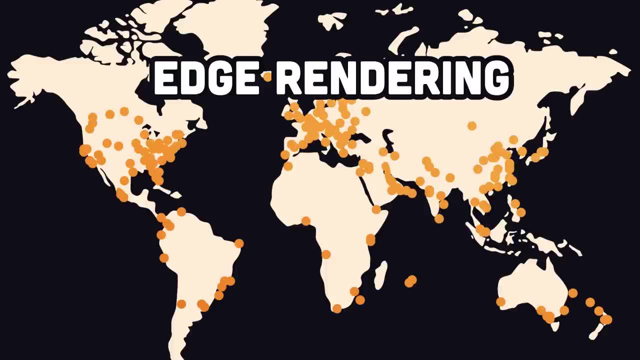 then JavaScript takes over to handle all subsequent navigation client-side. However, if that's not ideal, developers can set different rendering and caching rules for every route, and it's capable of running on edge networks like Cloudflare. Its built-in dev tools are: 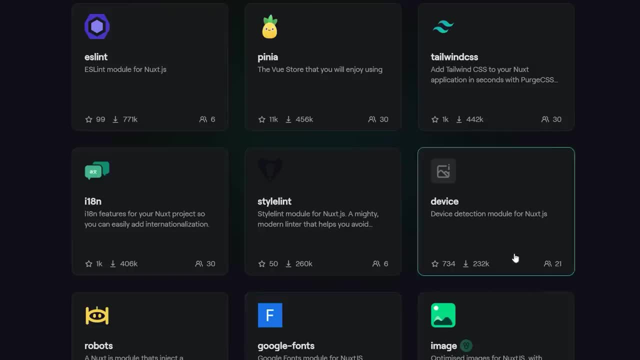 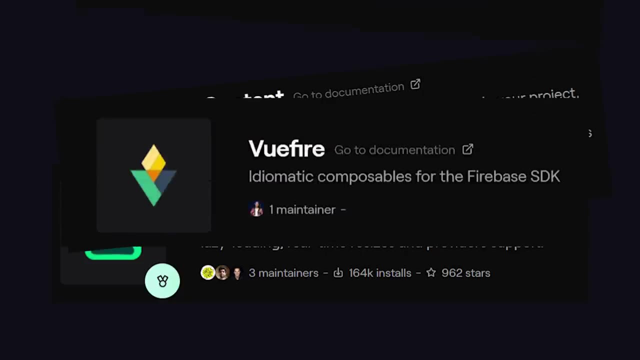 incredible and may trigger jealousy if you use a different framework. Beyond that, it has a huge ecosystem of modules that can handle requirements like image optimization, content management, database integrations, e-commerce and countless others. To get started, generate a new project with a CLI. then you'll find the main entry point in the appvue. 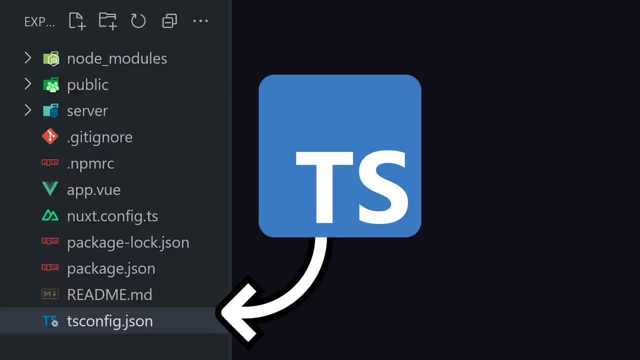 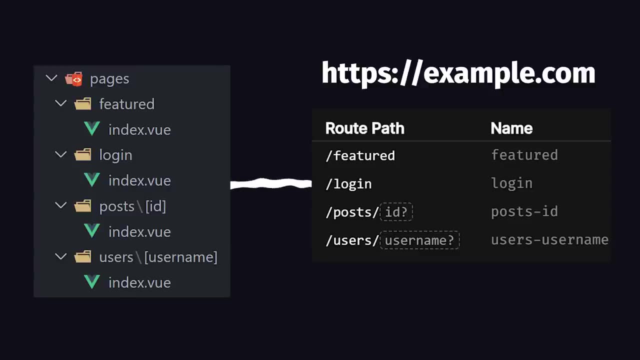 file And notice how it's configured with TypeScript out of the box to ensure your own safety. To build an application, you write Vue components in the pages directory. The structure of the file system determines the routes and URLs in the browser. What's unique about Nuxt, though? 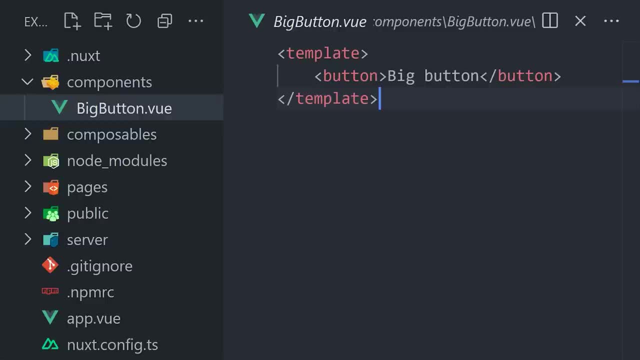 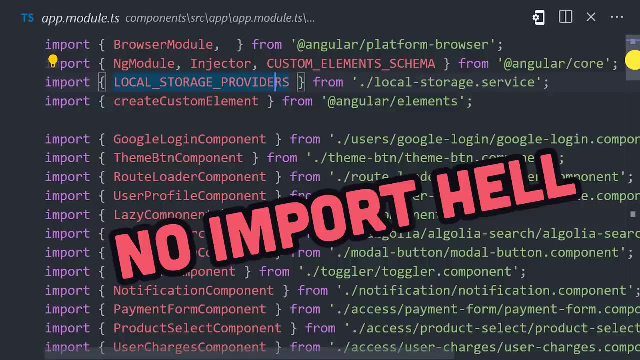 is that reusable components and composables have their own dedicated directories. Any code defined here can be automatically imported in your pages, and that means you don't need a massive list of import statements in every single page And under the hood, it will automatically. 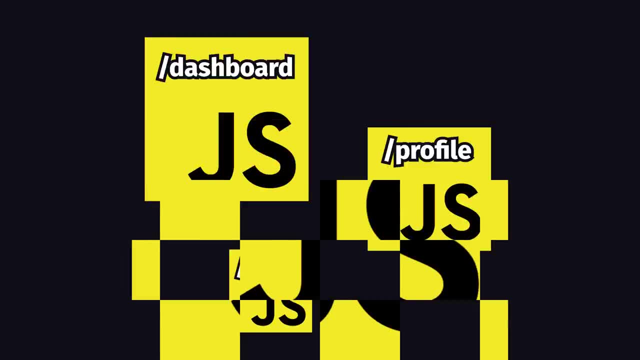 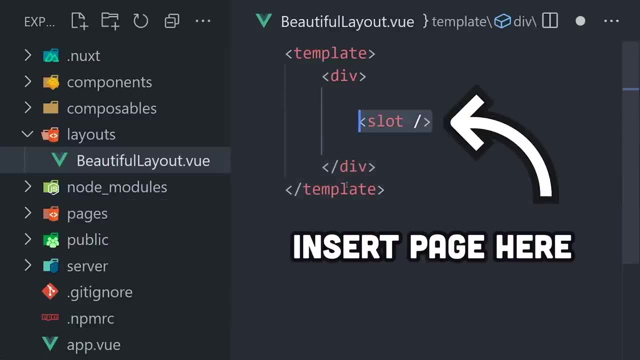 handle code splitting, so only the JavaScript needed for the components in this file will be sent downstream to the browser. Next up we have the layouts directory. Here we define Vue components that have a slot in the middle, allowing the outer UI, like a nav bar and footer, to be shared across. 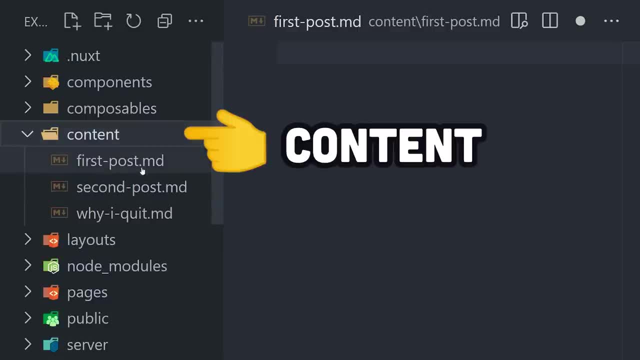 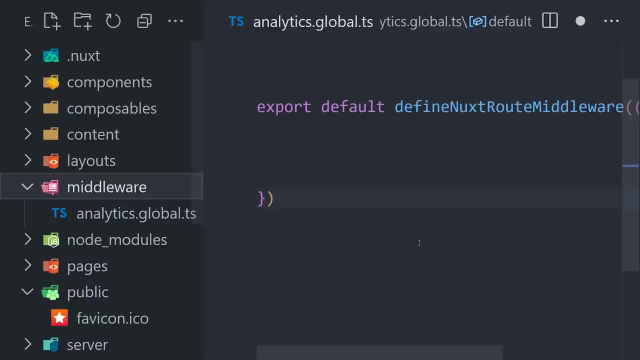 multiple pages. Now, if you're building a blog, you'll really like the content directory, because here you can write content in Markdown and use it throughout the application with minimal friction. Then we have the middleware directory, which is capable of running code. 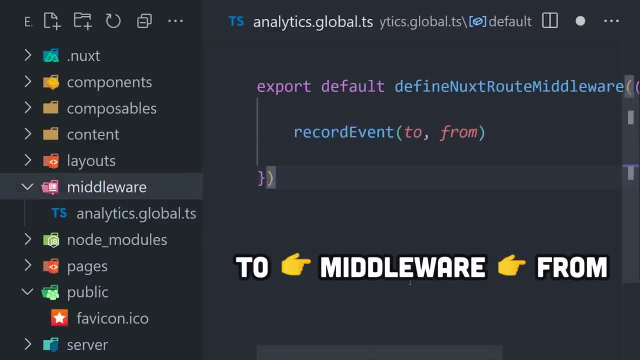 before you navigate to a route like for collecting analytics or checking the user authentication state. Nuxt has many other special directories to offer, but everything in the framework is progressively enhanced, which means you can update it every time you need it. You can. 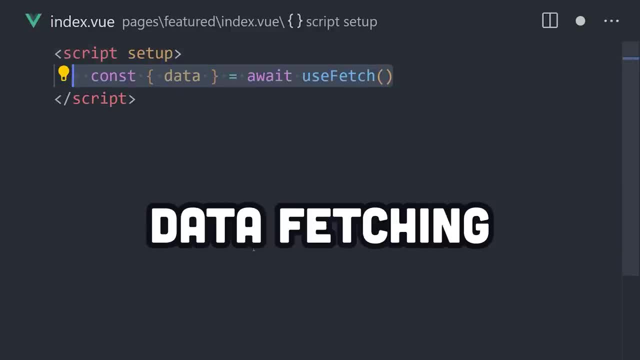 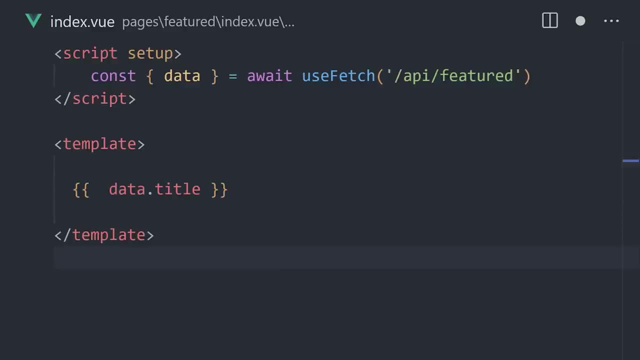 opt into these features as needed. Now, when it comes to data fetching, it has built-in composables like useFetch. It's built on top of the Fetch API in the browser, but can also cache and dedupe requests to make your application more efficient with zero effort. On top of that, it also provides a.